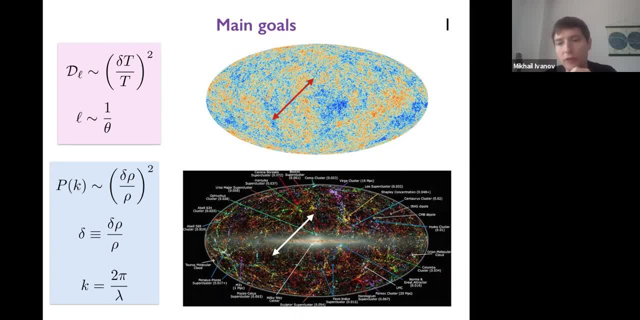 the multiple number And the shape of the CMB power spectrum is a function of sorry cosmological parameters. So now you can fit your model to this data and get the estimates for the parameters of our universe. A very similar picture takes place for a flash case structure. 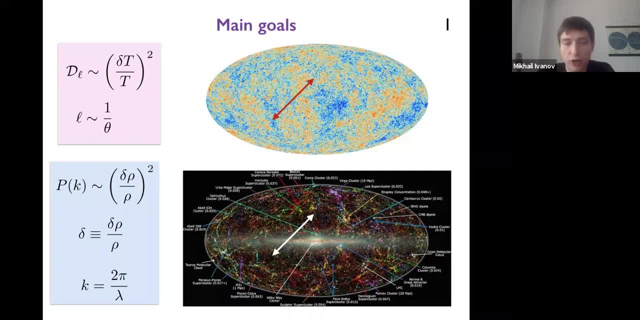 There, the galaxies represent the fluctuations of the density field, And this density field is observed on the sky. But, unlike the CMB, you can also measure the ratio to the galaxy And this way, in fact, you're dealing with a three-dimensional volume of data. You're dealing 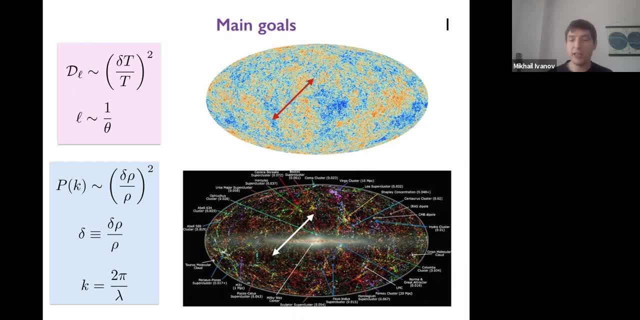 with the many images of the CMB, in some sense many images of the universe, which essentially allows you to get to measure the density distribution as a three-dimensional function, which now is Michael Well, the wave number is k Here, and also the shape of the galaxy power spectacle as a function of k is a function of cosmology and I can get the measurements of the molecule parameters from in. 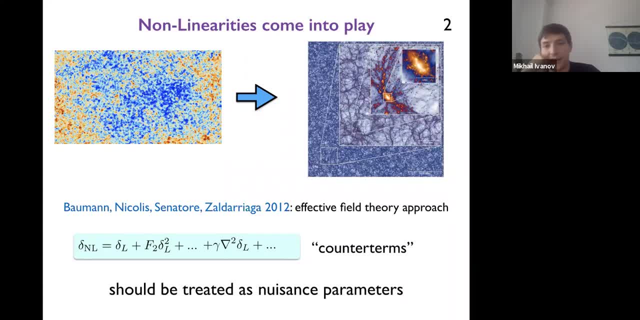 course, the complication behind this simple story is that the distribution of galaxies is very nonlinear, And here it's instructive to first take a look at the CMB. So if we look at the CMB map, then we'll see the Gaussian distribution. 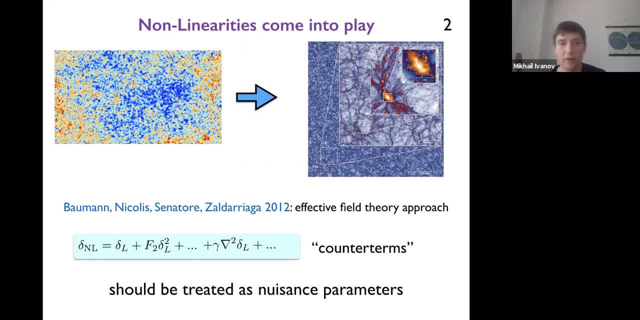 random distribution of cold and hot spots, more or less equal probability of high in the cold or cold spots, And then if you keep zooming in, if you go to shorter scales, then you'll see essentially pretty much the same picture, which essentially tells you that the distribution 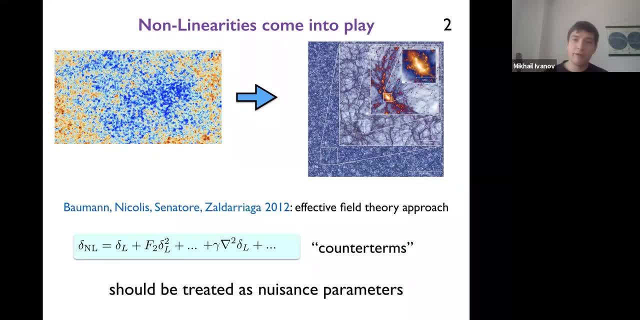 is Gaussian and it can describe a linear theory. However, for galaxies this is not the case And, of course, on large scales, the distribution of galaxies looks like CMB. It looks like a random distribution of overdensities and non-densities. 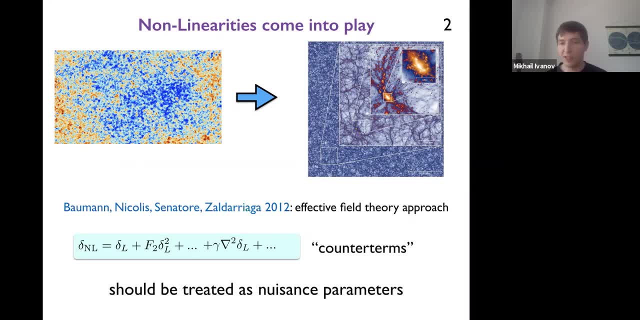 But as you keep zooming in you will start seeing some complicated structures like filaments, galaxy clusters and so on and so forth. So the field becomes very nonlinear and non-Gaussian. The theoretical description of nonlinear galaxy formation: the linear structure formation. 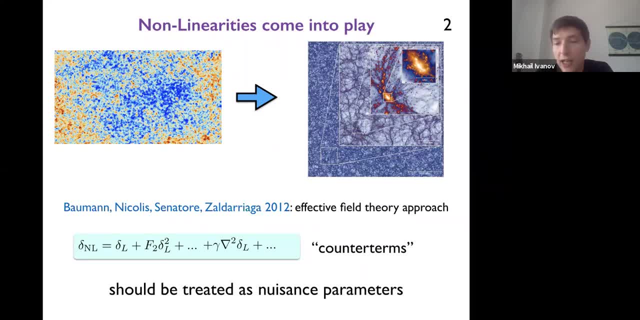 has been a matter of intense investigations for many decades And in that it has led us to the creation of the effective filter flash case structure, which was put forward roughly 10 years ago, And this theory provides a fully consistent mathematical description of the galaxy formation. 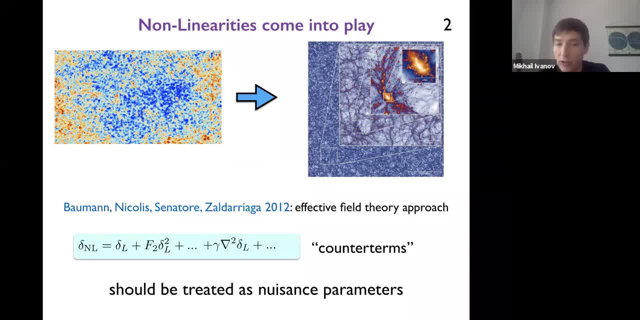 in the perturbative regime. So the nonlinear density field can be unambiguously mapped to the linear density field, which was the seat of structure formation 잖아요. And most importantly, this relation, this Taylor expansion, if you want it- involves some three coefficients which were called counterterms, and you should think of them as some effective parameters, like the viscosity for normal fluids, because we know that viscosity is generated by complicated molecular processes, but in large scales it's just one number, so you don't need to worry about this process. 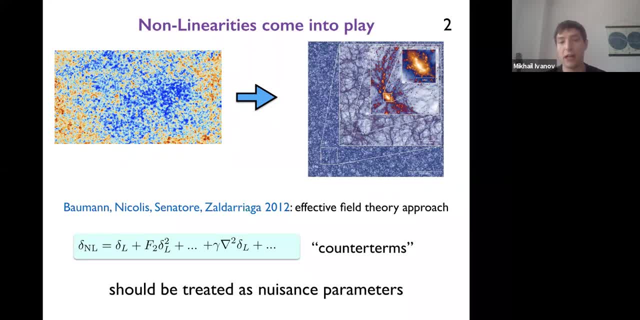 And the very same situation takes place for galaxies. so, even though the formation is very complicated on large scales, all the properties of this complicated physics can be encapsulated in a finite number of coefficients, which are called counterterms, and those should be treated as nuisance parameters in a data analysis. 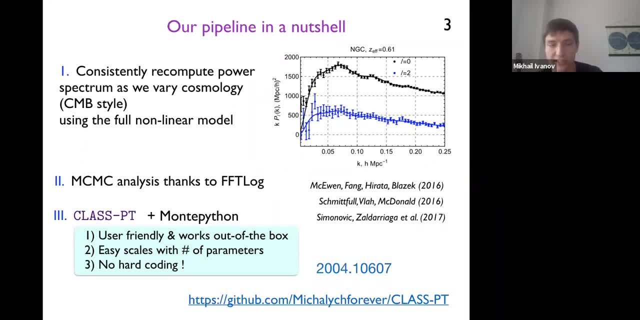 All right. so there has been this progress in the effects of filteria in other aspects. Now we have fully agreed how the nonlinear description should look like. Let's apply this to the actual data. Let's try to measure the cosmological parameters using this theory. 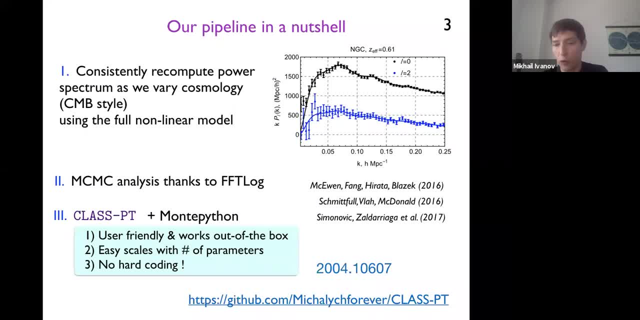 And this took us the creation of a whole pipeline from scratch. and the main idea behind this pipeline is to be able to consistently recompute the power spectrum, the nonlinear power spectrum, as the very cosmological parameters in the CBA style. So would you? 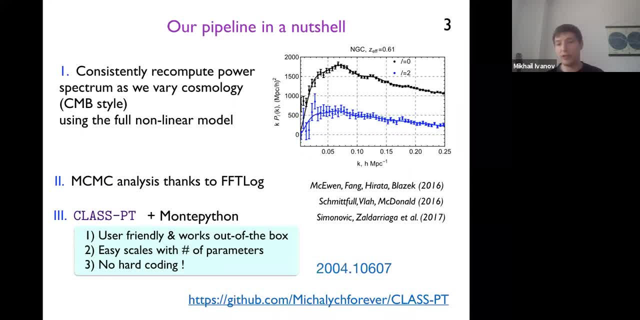 So we define a model, say one the CDM, and then we fit the parameters. for a set of parameters of this model, We compute the shape of the matter-power spectrum and fit the theoretical predictions with data, just like we do for the CMB. 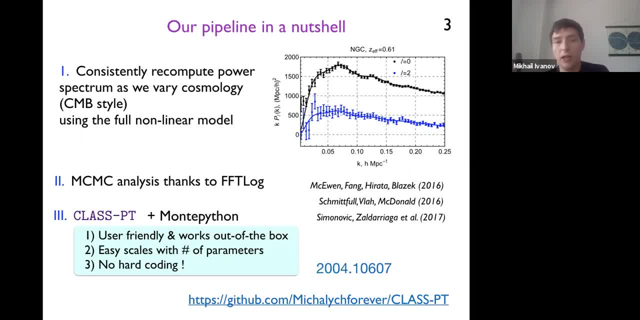 And of course, given that this calculation is nonlinear, it's more complicated than just running usual Boltzmann codes. So also it took a lot of effort to be able to efficiently carry out this calculation. and in particular here we're using the FFT local algorithm, which allows for fast and efficient calculation of the nonlinear power spectrum. 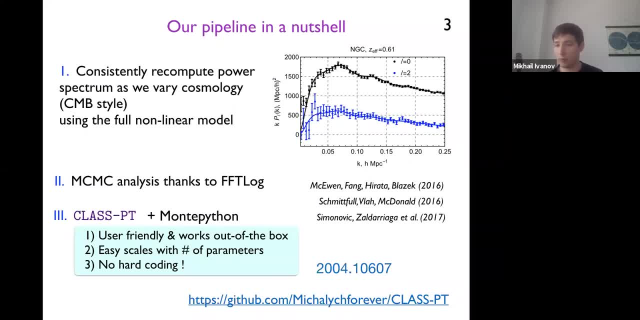 And now we have put all these ingredients, the full nonlinear power spectrum with all the contractors, bias parameters, all the theoretical features. we have put everything together in a code called ClassPT. This is an extension of the standard Boltzmann code class which can be interfaced with standard MCMC samplers like 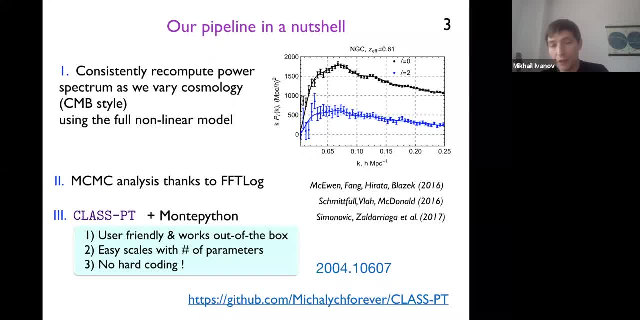 Montepython so that you can take advantage of the virtues of this combination. It's very user-friendly. you can easily include new parameters in the model. you can explore various beyond-standard model scenarios. it doesn't require any hard coding. 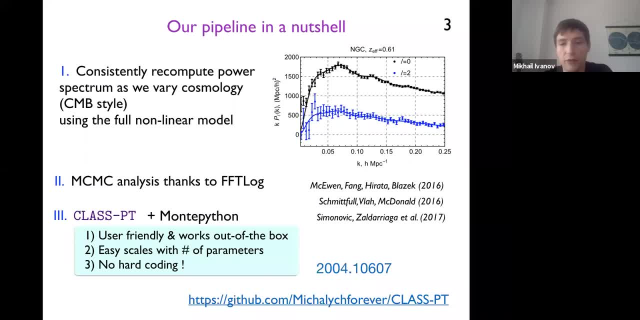 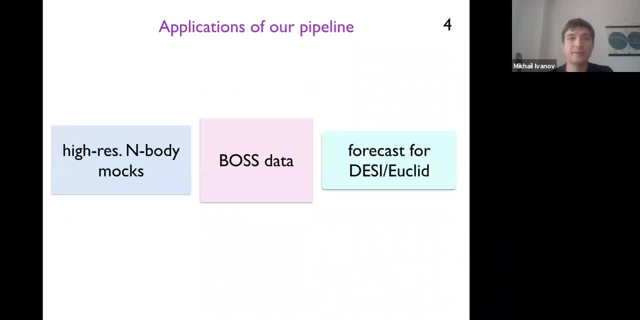 If you know how to run Class and Montepython, then it should be easy for you to run our extension as well. So you can find our pipeline online, please, you're free to use it. Now I'm going to discuss three different applications of this pipeline. 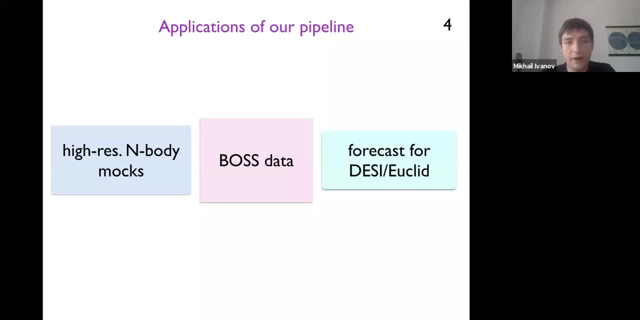 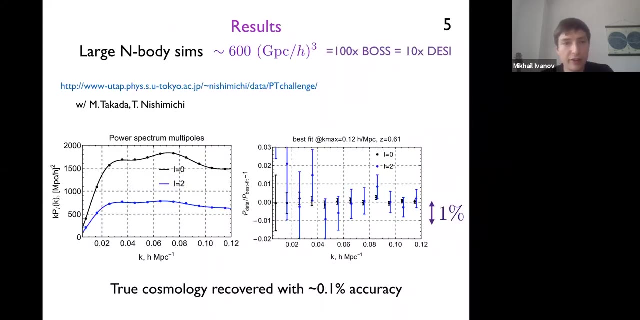 First, it's validation with high-resolution body simulations. second, the application to the actual BOSS data. and third, I will discuss a forecast for future surveys like DAISY and Euclid. So once we have created our pipeline, we validated it by participating in a blind challenge organized by Masahiro Takada and Takahiro Nishimishi. 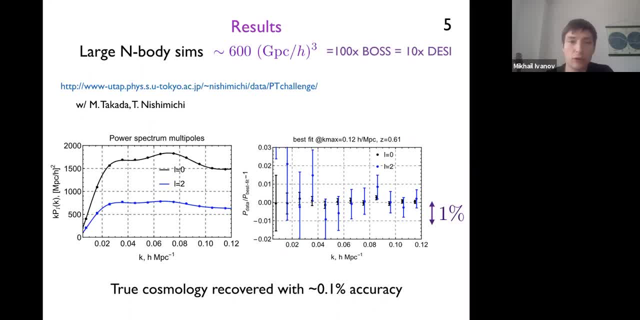 So they have run a large suite of in-body simulations with the total cumulative volume 600 gigabyte per second. So we have a total of 100 times the BOSS volume, or 10 times the volume of our climate surveys like DAISY. and all this data is available online. 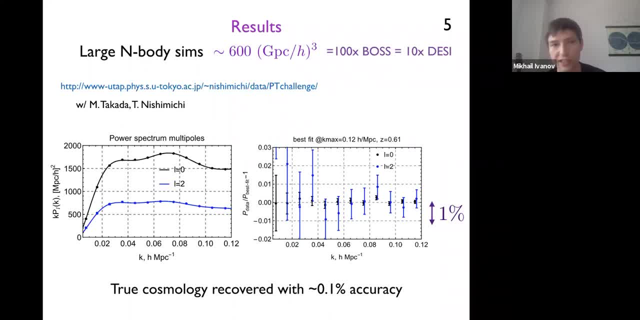 So essentially Masahiro and Takahiro, they have run these simulations and have measured the galaxy power spectra that corresponds more or less to the BOSS galaxy sample and gave us this spectra but didn't tell us the correct cosmological parameters that were used to generate all spectra. 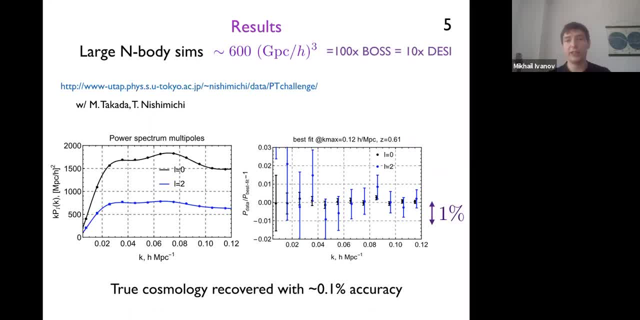 And the task was to actually measure them. so we applied our code, well, applied our model and just fitted this data. So here on the left you can actually see this data, you can see the monopole and the quadrupole moment of the galaxy, of the retro space galaxy power spectrum. 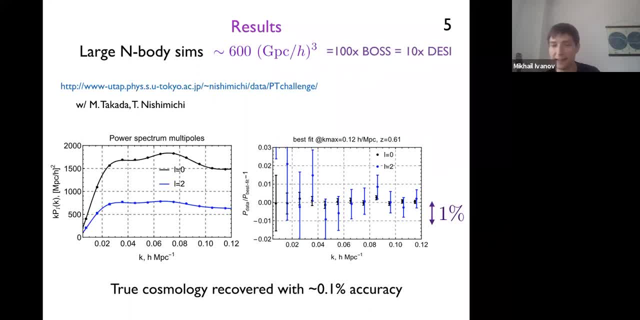 So here I just remind you that the monopole is the galaxy density auto power spectrum, and the quadrupole should be thought of as the cross-correlation between the galaxy density and the galaxy velocity field. So this is the data that you get to observe thanks to retro space distortion. 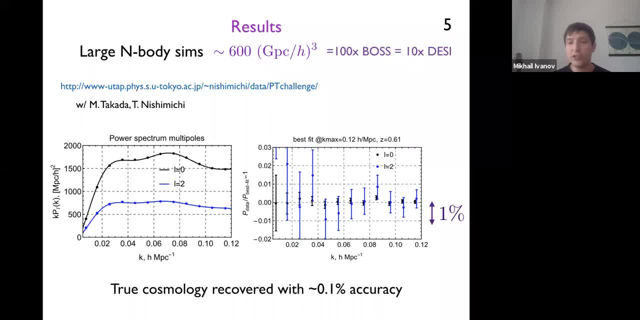 distortions and it's very important that the BOSS distribution is unbiased on large scale, so there is no galaxy bias and you get to measure the linear clustering amplitude without paying the price of galaxy biasing for this observable. Alright, so here you can see the data. on the left, you see the data points. you don't see the error bars because they're super small, they're 0.1%. you can see them better on the in the right side, in the right part of the figure. 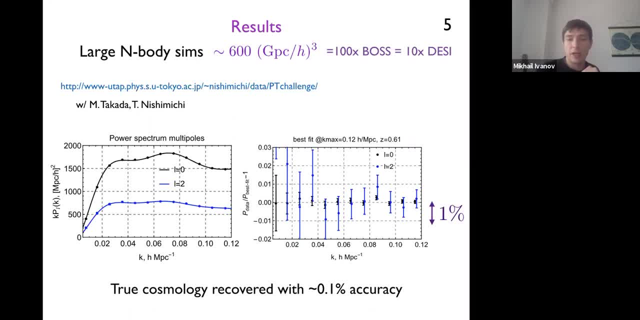 So you see the residual between the data and the best fit, and really we can fit, our model can fit the data to 0.1% precision within this crazily small error bars. And here maybe, yeah, I should say that not only it's able to fit but also the optimal parameters that we get from our analysis. really they within the error bars corresponding to this huge volume, they correspond to the true cosmology, so we're able to recover the 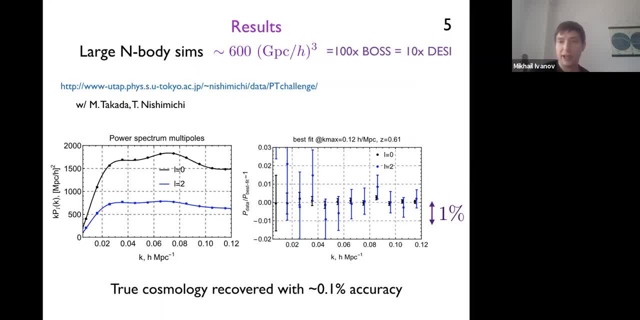 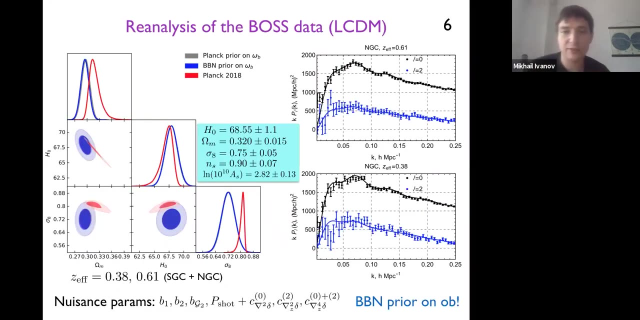 true cosmological parameters with 0.1% accuracy from this large simulations. And after that we got confident in our pipeline and decided to apply the actual BOSS data. And essentially we have done, we have repeated the same exercise, we took the available galaxy power spectrum measurements from 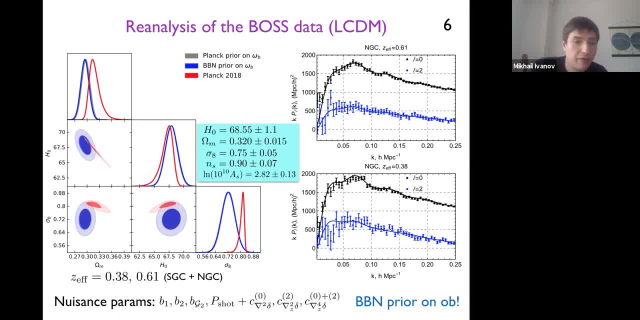 essentially four non-overlapping BOSS data chunks at effective ratios 0.38 and 0.61.. Two different factors of the sky: south galactic up and north galactic up- And, having fixed the model to be based on the CDM, we fitted the parameters of this model to the data and 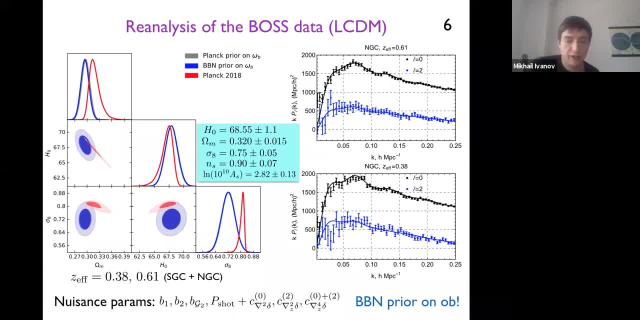 having fixed the BBM prior on omega baryons, on the physical density of baryons, we're able to measure all the remaining parameters of lambda, CDM, including H-node and omega matter. So omega matter is the current abundance of matter and you can see that these two parameters 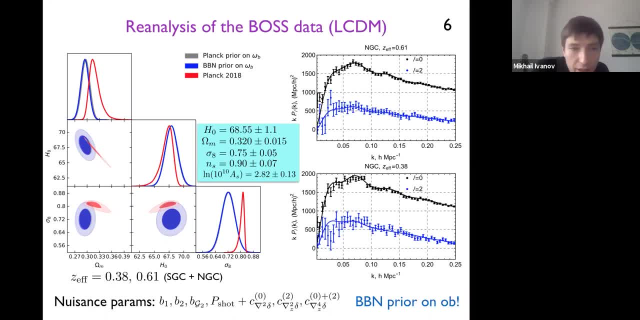 H-node and omega matter are measured as good as Planck. So here on the left panel you can see some portion of the posterior distribution of the corner plot from our MCMC analysis with, along with the Planck measurements, and you can see that really the BOSS data is very 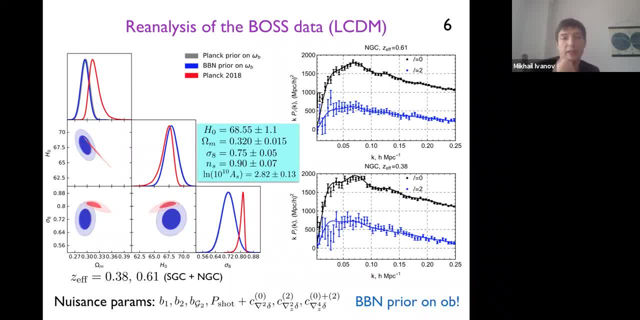 competitive with Planck in terms of H-node and omega matter. Then we're also able to measure other parameters like sigma a, the clustering amplitude, or the power spectrum, the tilt- the tilt of the primordial power spectrum, ns, and we have found that this parameter is very close to 1, which is consistent with the basic inflationist scenarios. So in other words, we've got some independent evidence for inflation from the BOSS data. 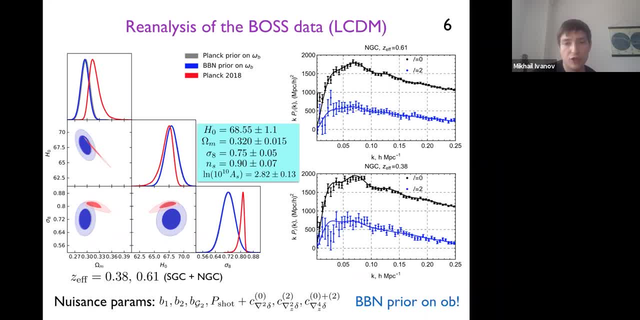 And also we're able to measure the amplitude of the initial power spectrum, which happened to be very similar to the Planck prediction, although with larger error bars. Here maybe I should point out that we in all this analysis, we had fixed the model to be on the same when we used the deviant prior on omega-variance. but if you don't impose this prior, in principle you can perform the same measurement. you can measure omega-variance from the shape of the galaxy power spectrum. 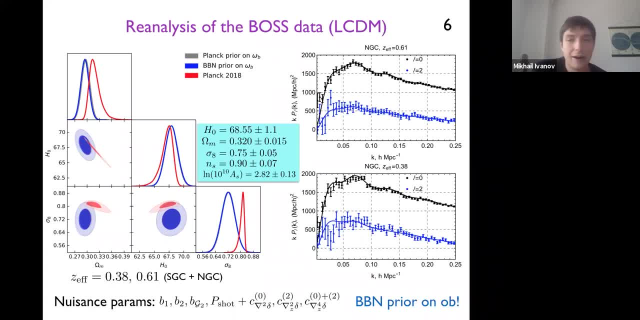 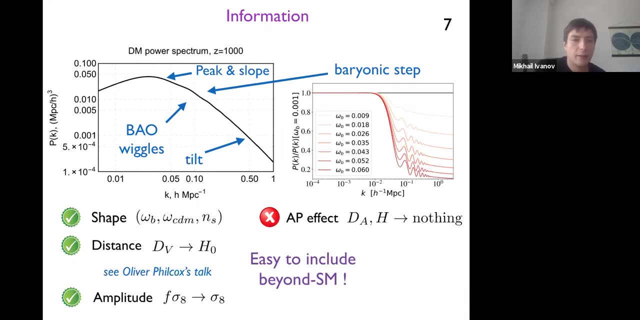 And this way you can derive the constraints on H-node that are independent of the sound horizon, and I think that Oliver Philcox is going to talk more about this in his talk. All right, so where all this information came from? Here in this slide in the left panel, you can see the matter. power spectrum attracted to 1000 after a combination. 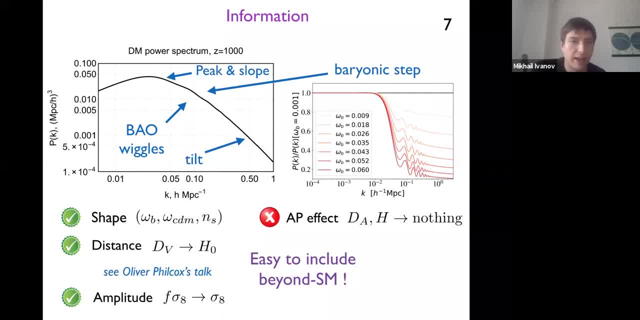 as a function of the wave number. you can see that this power spectrum has a very non-trivial shape. it has a turnover, it has some interesting slope. Also, of course, there are Biot-Wiggles which we won't know. then. 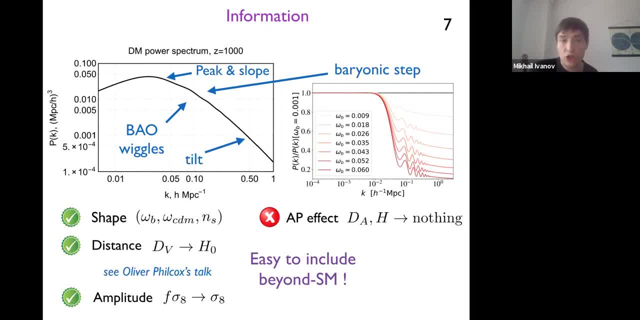 this is characterized by some tilt which is not disjointed with the slope, and another feature is the so-called baryonic step, which is generated by the baryon's free-streaming before a combination. And essentially all these spectral features. they are sensitive to the so-called shape parameters like omega-variance, omega-CDM, NNS that can be measured. 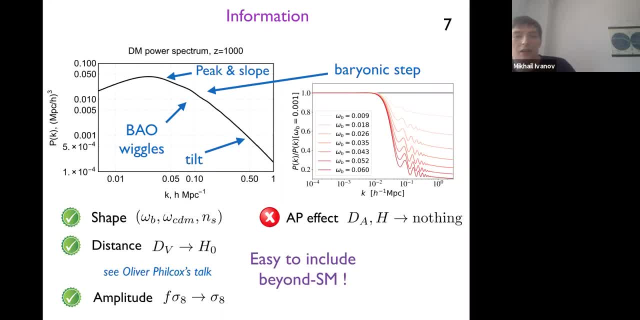 from the shape of the power spectrum, regardless of any distance information. And once you know this shape parameter, just like in the CMB, you have the estimates for the features in the power spectrum and then you can convert the observed angular size of these features into the distance. 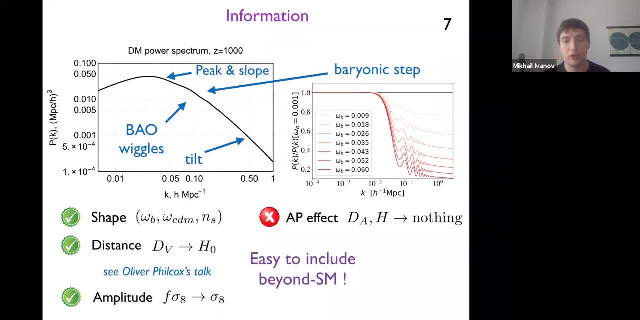 The angular size into the distance using the absolute size deduced from measurement of these parameters, So you can get the distance measurement. In general it is sensitive to the so-called volume average distance dv, But in lambda-CM it reduces it just to h-naught. 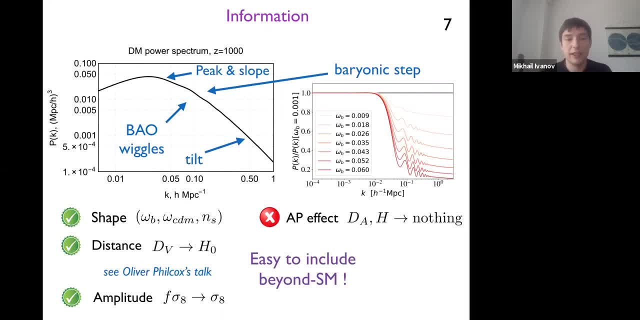 This is how you get to measure h-naught from the galaxy power spectrum, and I think that Oliver is going to talk more about this. And then in lambda-CM, the amplitude of the power spectrum is characterized by the combination f-sigma-8, because, as I told you, 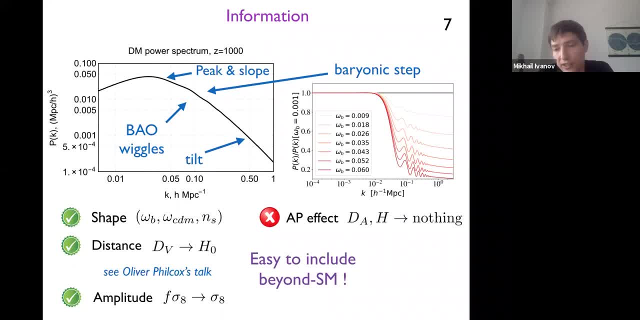 only the velocity field is unbiased and the velocity field is characterized by f-sigma-8,, but then f is a derived parameter, is entirely fixed by h-naught and omega-matter in lambda-CM, such that you get to measure sigma-8 without f and this you can convert into the primordial amplitude as having assumed a model like lambda-CM. 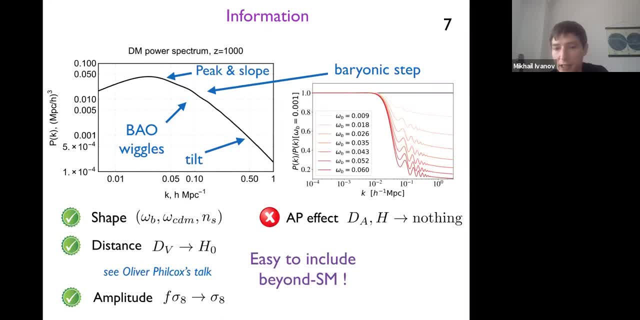 Then there is another effect which is unique to galaxies- It's absent for the CB- which is the Al-Khapachinsky effect, and it has been the main probe of previous Laschke structure. full-shape analysis: In principle, it allows you to measure. 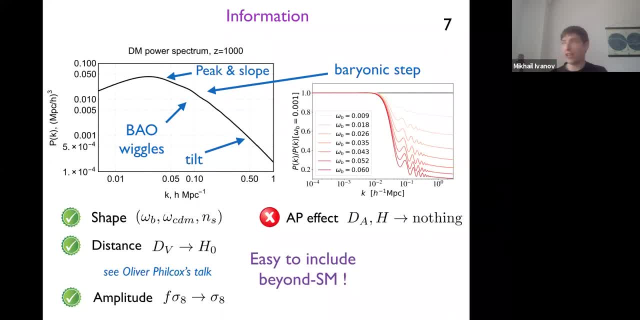 in a model-independent way the angular diameter distance and the radial distance of the galaxies. but those measurements are not very precise and in lambda-CM for instance, they give no extra information to you. But of course in the extensions of lambda-CM this effect can be important. 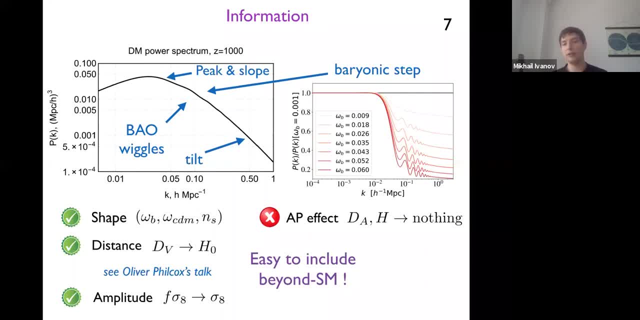 So I have presented all the discussion for lambda-CM, but you can imagine that all these arguments can be repeated for any beyond-the-standard model scenario, For instance if you want to change the early physics. and here maybe I should also mention that the standard analysis uses the. it fixes the. 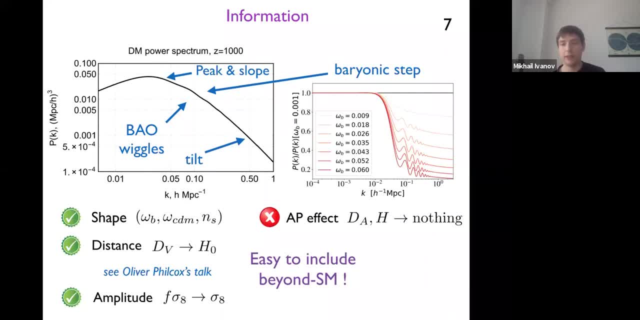 shape the power spectrum shape template in and then applies only the Al-Khapachinsky distortions to it, which means that in principle the standard full-shape measurements, say by Bose, they cannot capture the scenario that modify the early universe, And one of them is early dark energy. 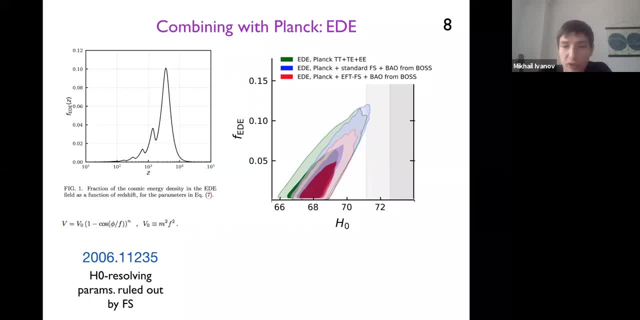 Maybe you know that this is a very popular scenario which has been put forward to resolve the so-called Hubble tension And essentially the idea behind this scenario is that if you had some axiom-like scalar field prior to recombination and this scalar field 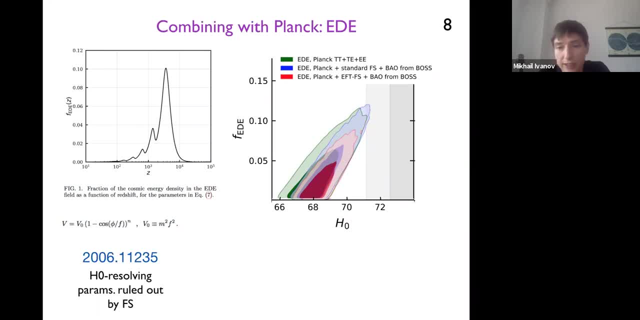 contributed to 10% of the total energy budget at this epoch, then it would be enough to reduce the size of the Sun horizon and then maintain a good fit to this Planck CMB data, while simultaneously agreeing with the local H0 measurements. But 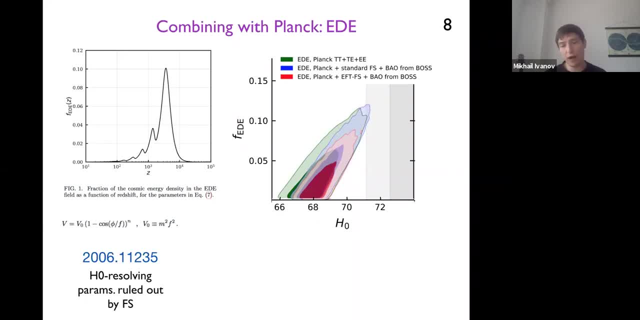 however, maintaining a good fit to the CMB requires shifts of other cosmological parameters and those shifts are intentioned with the Lascaux structure data with the shape of the galaxy power spectrum. So we have done a joint analysis of the early dark energy scenario using the Planck CMB data and the 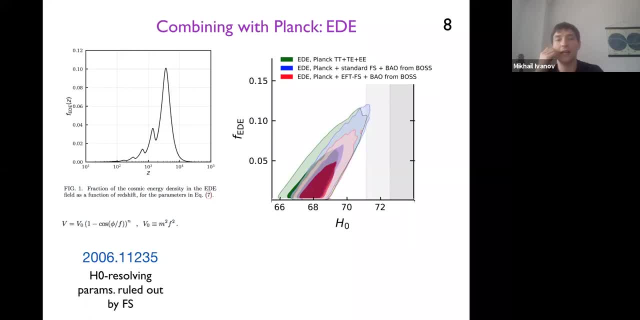 Bose full-shape measurements, and we have found that, indeed, the parameter, the region of parameter space that resolves the Hubble tension and which is not strongly excluded by CMB, becomes disfavorable once you include this data, In other words the early dark energy scenario. 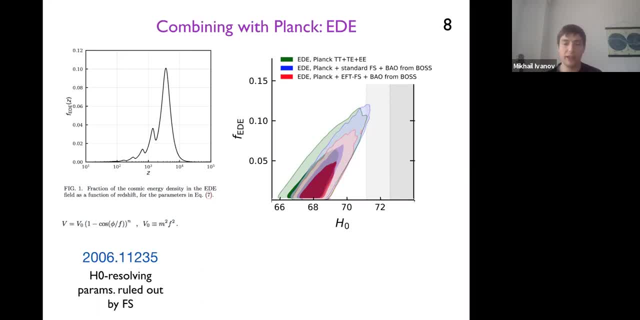 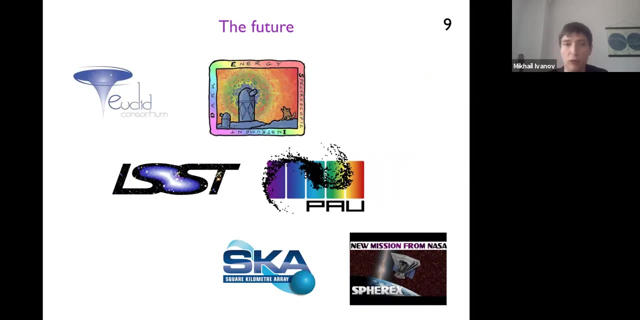 which resolves the Hubble tension. it fails to simultaneously fit the shape of the matter power spectrum which allowed us to derive the strongest constraint on this scenario to date. All right, let's discuss the future, because we know that there are many Lascaux structure surveys coming online in the 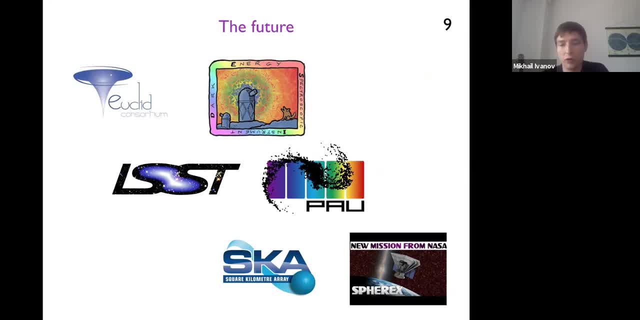 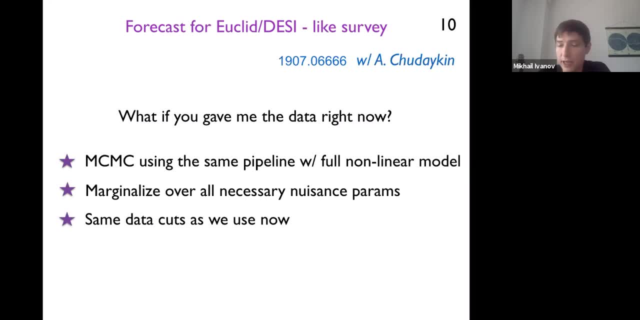 coming years. so, like Euclid or DESY, and we have done a forecast for this survey, trying to understand what kind of error bars are we going to get from them on cosmological parameters. And I guess the main idea of this forecast was: 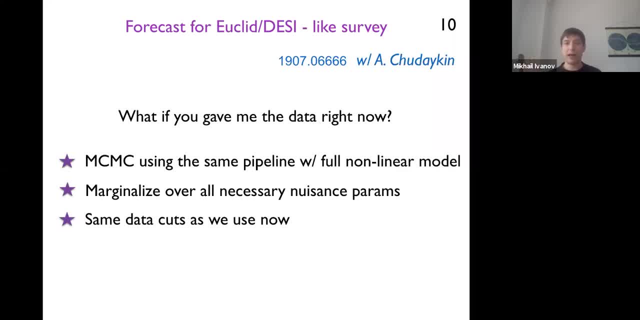 the following: What if we apply? what if you gave me the data right now? Because we have already the pipeline, we have everything. So what if you gave me that right now? What would be the constraint? So we don't need to build any extra infrastructure. 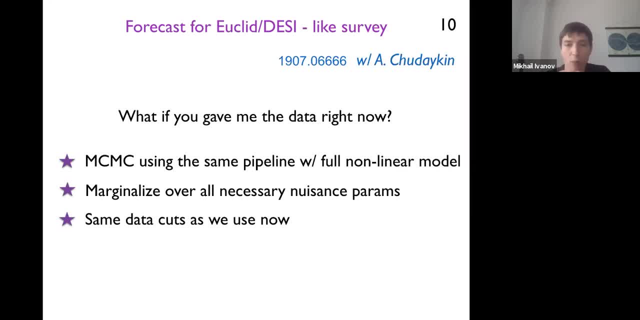 So to answer this question, we have generated the mock Euclid data from the spectroscopic specification available in the literature and we have run the full MCMC analysis of this mock data using the full nonlinear model and having marginalized our own necessary nuisance parameters. 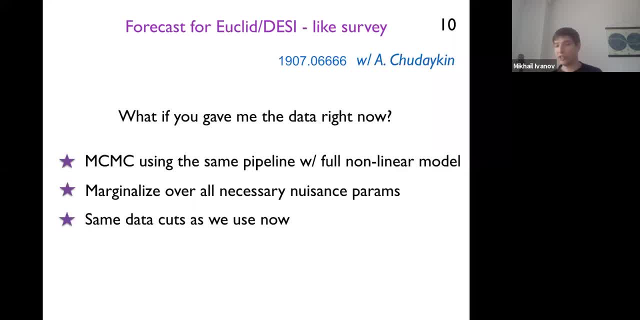 And then we use the same data cast as we use now. So we decided to be very conservative in a sense, because of course there are many years to come and maybe in these years we'll be able to make some progress and make even more improvements. But however, even in this very 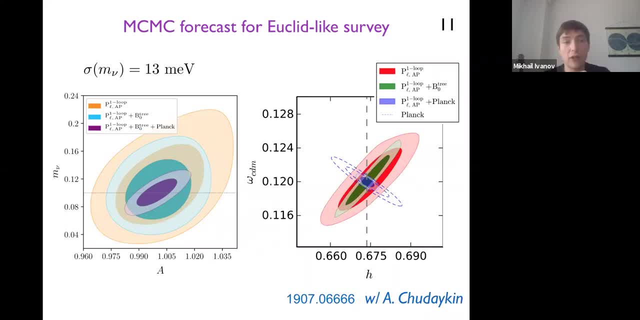 conservative scenario, we're able to get very strong constraints on the neutrino mass. So here on the left plot I'm showing you the posterior distribution of the neutrino mass versus the amplitude, the primordial, the amplitude of the primordial power spectrum, which is very. these two parameters are very degenerate. 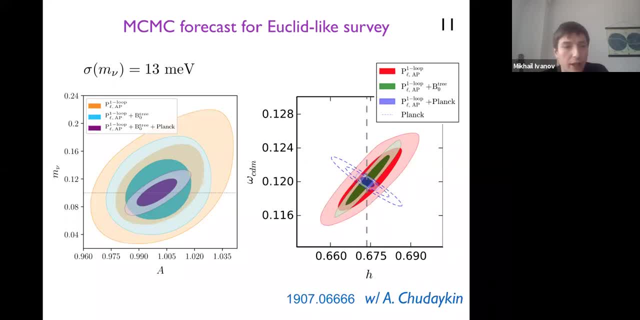 But, however, with the future service, using only the power spectrum data alone, you'll be able to break the degeneracy and measure the neutrino mass to precision like 30 milli-electron volts from the power spectrum shape alone. Then if you combine it with the bi-spectrum data, in principle you'll be able to reduce. 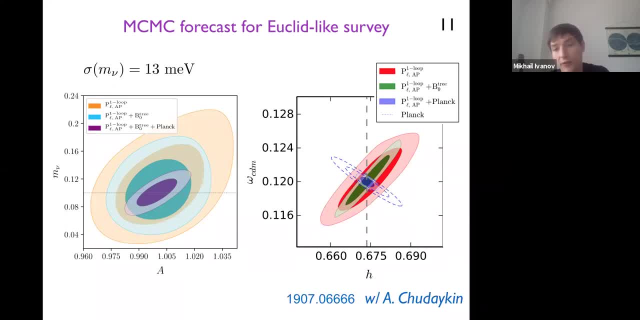 the error bars by 30 percent, down to something like 20 milli-electron volts And, of course, when you combine the full wash structure data with Planck, you'll be able to get the final constraint, which is the one sigma error bar, equal 13 milli-electron volts. In other words, you'll be able to: 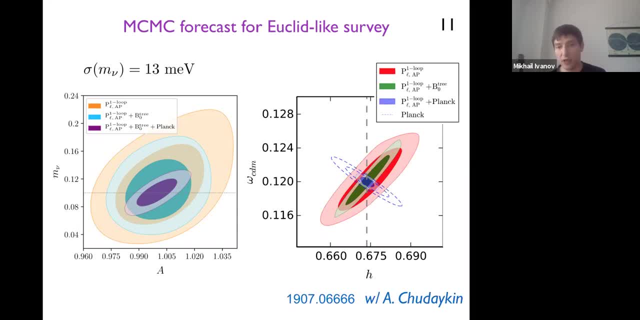 measure the minimal guaranteed neutrino mass at five sigma level. And also, as far as other cosmological parameters are concerned, you'll be able to measure them from the power spectrum data alone, as good as from Planck. And, importantly, these measurements will have different contour orientations so that when you combine 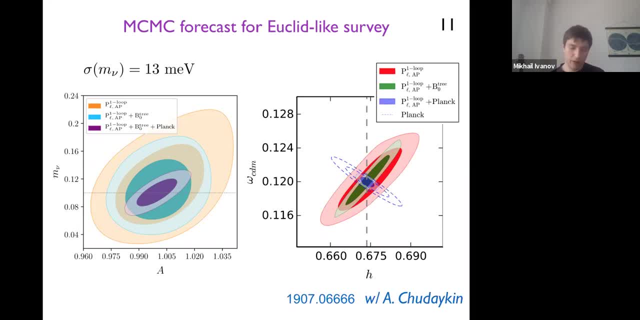 the contours, likelihoods from Planck and the likelihood from Euclid or Dessy, you'll be able to massively break these degeneracies and get super tight constraints on the cosmological parameters of Lambda-CTM, For instance, for each node you will be able to get a 0.1 percent. 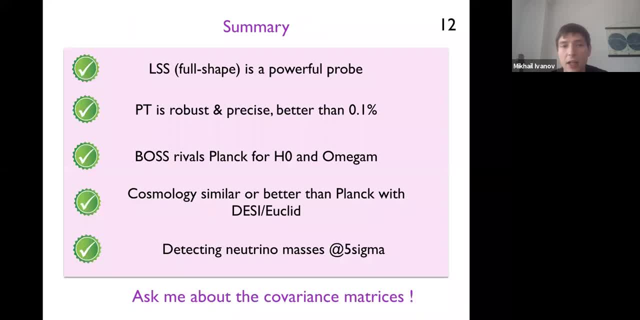 precision measurement. All right, let me summarize. I hope I have convinced you that the full shape of the galaxy power spectrum is a very powerful probe, And it already gives you some interesting results and new information about our universe. All this was possible thanks to the